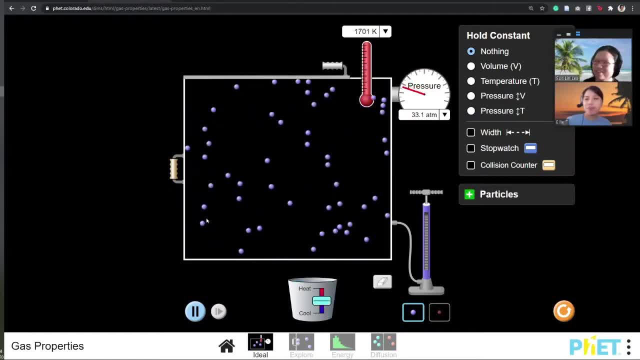 if we want the particles to move faster. I guess another method is to change the volume of the container. Do you think we should give them more space to move or less space to move? Let's see. Let's say I increase the volume or the gas expands. 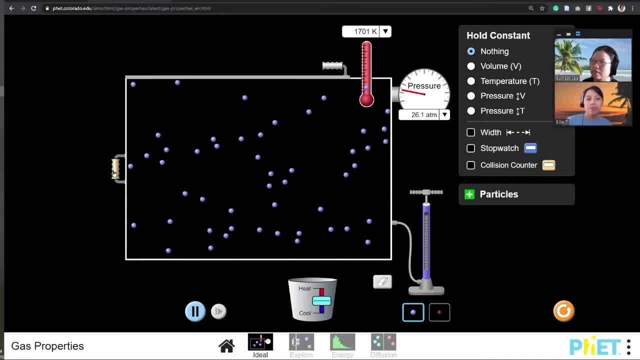 You can see now that the gas is traveling kind of slower, right? Okay, so remember this movement And then now I'm going to compress the gas All the way, All the way, And you can see that now we have much more energetic gases. 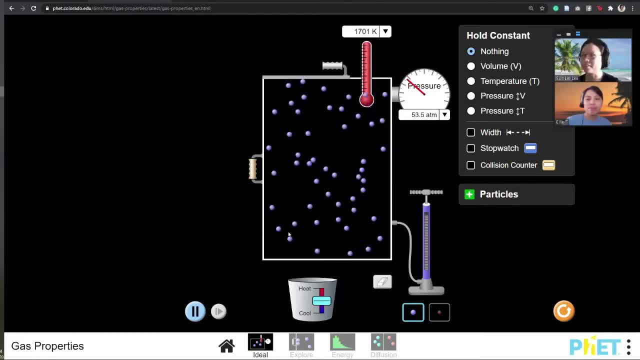 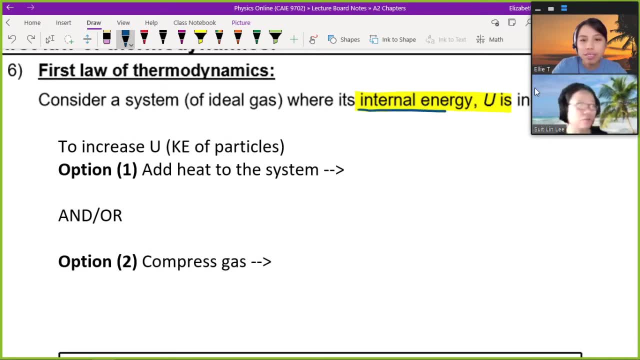 So there are two methods to increase the internal energy. Okay, so just now, when we look at the simulation, we wanted to increase the internal energy. So, as you mentioned just now, the most straightforward way is to add heat to the system. Okay, so we'll put a plus Q. 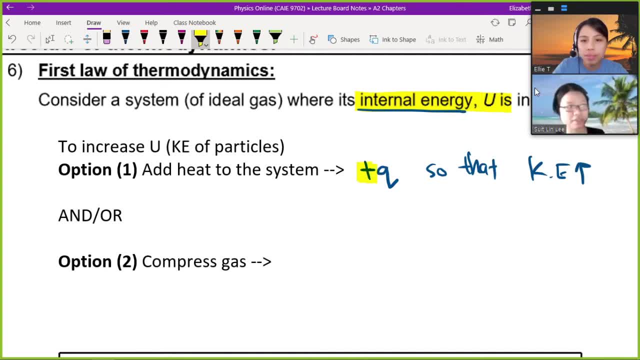 Okay, Okay, so that the Ke increases. But I want you to understand that just because you add heat to the system doesn't mean that the temperature of the system increases. There are special, special cases that we will look into later. But we can also add or compress the gas. 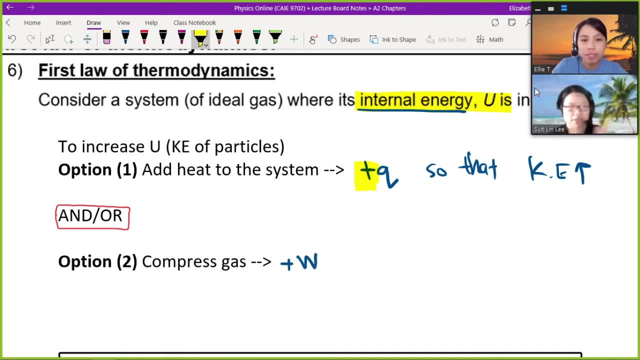 Basically giving the gas less space to move, So more collision with each other, So there's a higher chance for you to have a larger speed. So this one will be plus W, But this is less volume, Okay, So less volume here means work done. 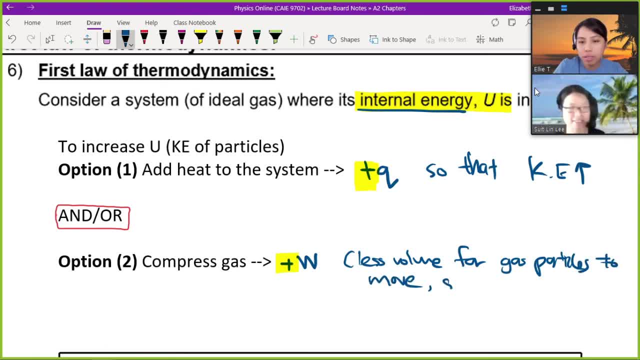 You compress on the gas, Right? So the whole idea here of internal energy is: we want kinetic energy to increase, And kinetic energy is the one that is related to heat. So kinetic energy is the one that's related to temperature, not heat. 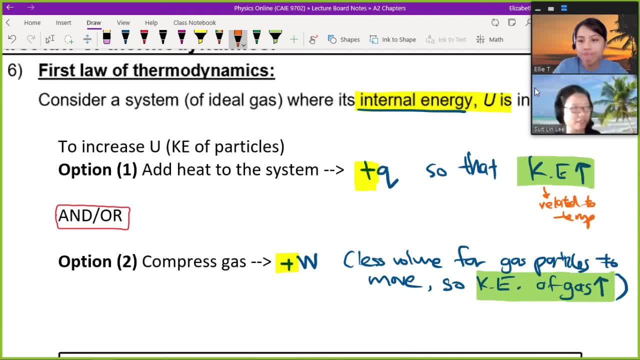 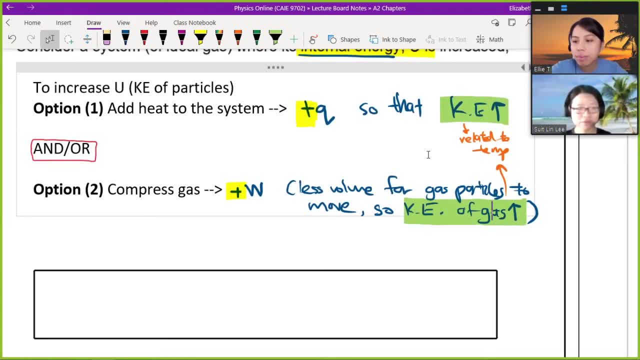 Okay, So I think we can think a little bit about conservation of energy here. To increase heat, To increase the internal energy, I have two options. I can choose either one or both. So I'll write: the increase or the change in internal energy will be equal to Q plus W. 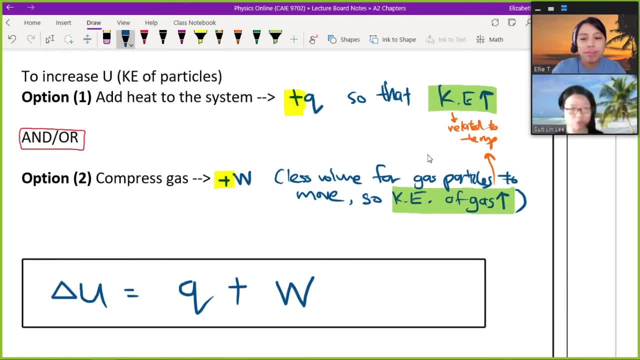 This conservation of energy is first law of thermodynamics And we will use this a lot in the following examples from this subtopic: Miss, got. second law of thermodynamics: got, Got, got, many many law, Got zero law. We don't care. 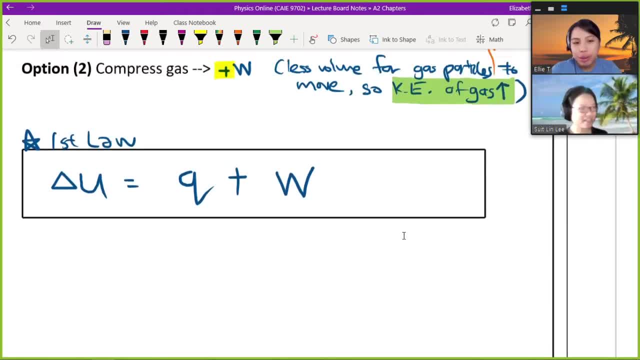 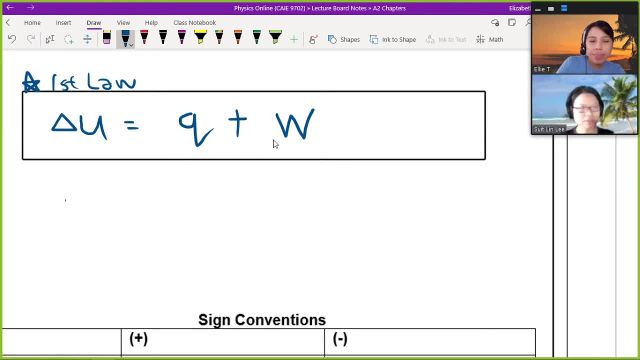 Got zero law, also Got zero law. Okay, Miss, I have a question. So how do we visualize this? UQW? ah, Is there a way? We draw a gas sample and then we think to ourselves: I want the particle to move faster. 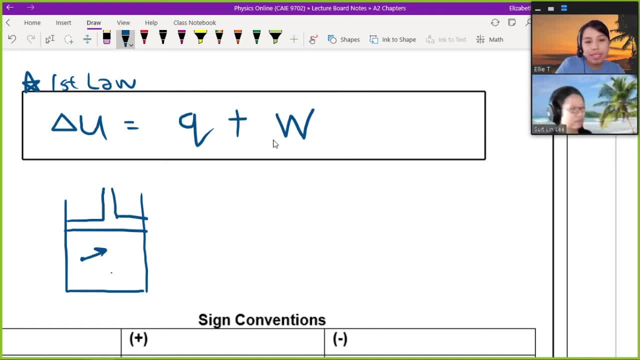 Okay, So maybe we imagine this piston thing. la Got particle fly high, fly there. Draw arrow to represent the speed law, because this is not a simulation. We don't. I don't teach in Hogwarts. I cannot put simulation in your notes. 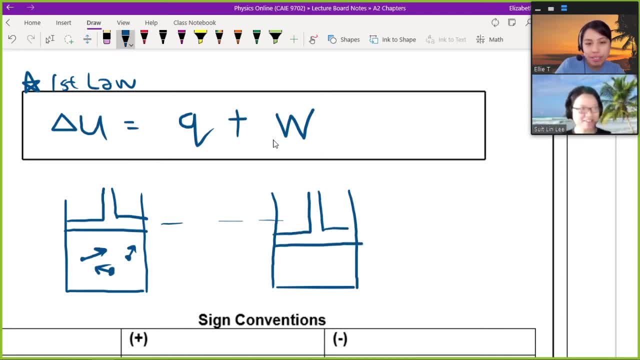 So if you compress this, then the particle will move faster. Wah, ding-dong-dong, ding-dong-dong. Yup, yeah, there we go. Okay, so I think I will write there that V decreases And because of this your W is positive. 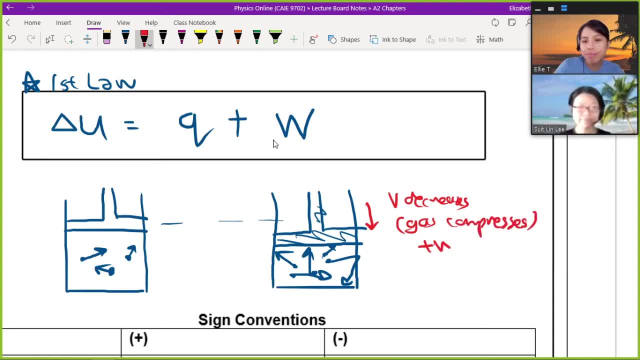 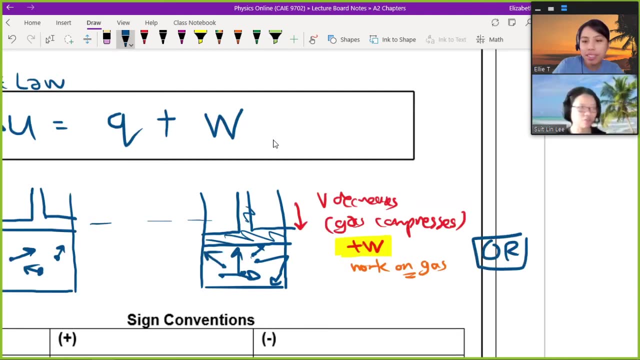 So you're doing work on the system. So it's either you using your hand to press down, or maybe atmosphere or changes in the surrounding does work on the gas. Okay, The chemistry of adding it is to draw two arrows underneath the gas lah. 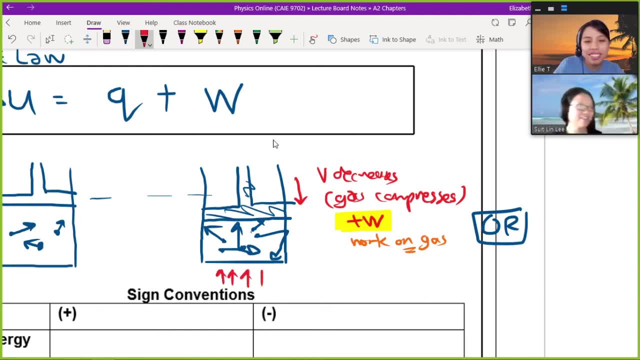 Heat lah. okay lah, I guess you could draw fire again. Never mind, we see a lot of fire already. Plus Q Or plus Q, Or both, Can do both. ah, number one or number two, Yeah, one or two, or one plus two. 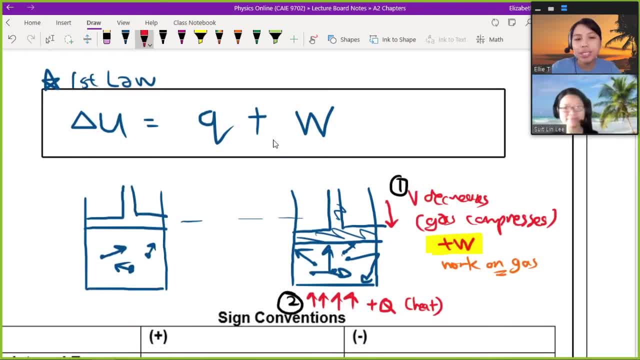 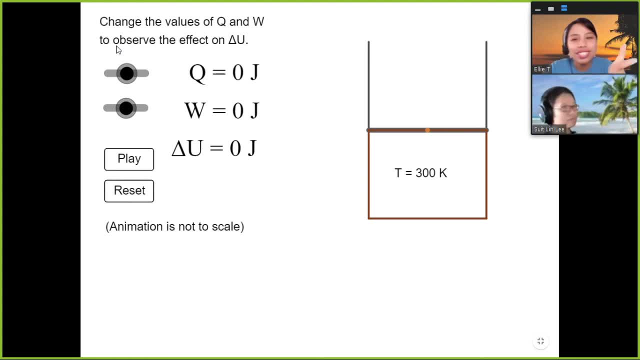 Oh interesting. So yeah, lor, I mentioned got simulation. Let me show you a very quick one. So here it's just basically showing you how you can see the values change, lah, okay, So you want to increase this delta U? What you can do is number one: you add heat. 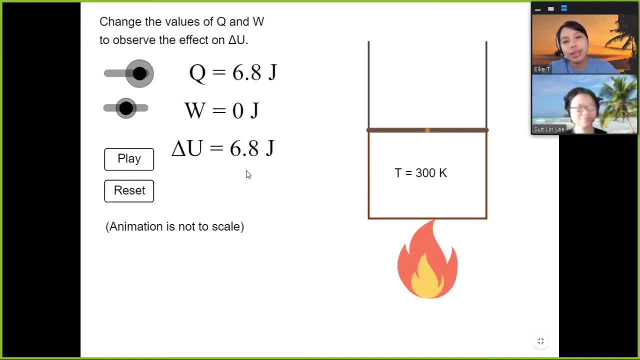 So you see, got fire come out: 6.8,, 6.8.. Okay lor, internal energy increased lah. But miss, miss, if W is zero, this means that the volume doesn't change. See, the piston didn't move. 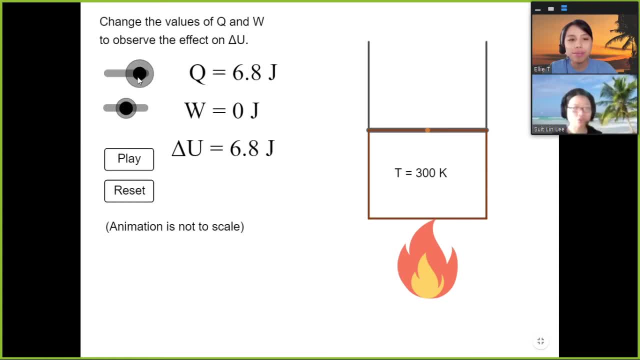 Still same volume, same box, So we can choose to just add heat to the system without allowing the gas to expand. So the container is sealed lah, Okay. Okay, the other one. ah. What if we Oh can play this one, ah. 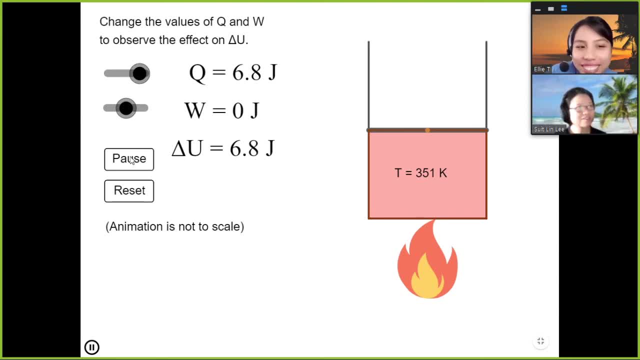 Oh, you can play. So you see, you get redder and redder and redder when you add heat, Yeah, and then it stays at a certain temperature, Okay, okay, What if we do work on the system? So you see the hand. 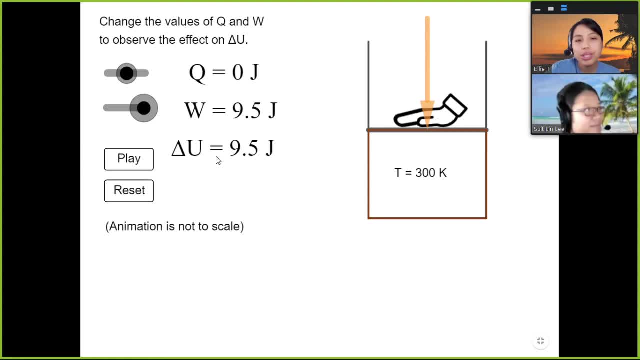 Press down on the gas. Hmm, So this will cause a increase in internal energy also, without adding heat. Changing, Yeah, Changing the heat. So, like that, lor, You squash it. you see it become redder and redder. Ugh, become very hot. 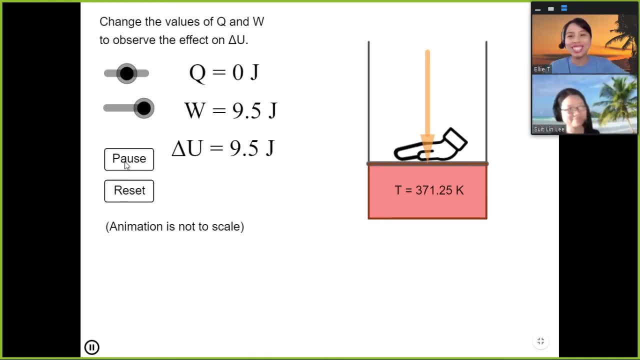 Hotter and hotter. Later we show you some video, very cool one. You can use it for survival in a while. Okay, anyway, So exciting. Okay, Then you can do one more where you Wow, what can we do? 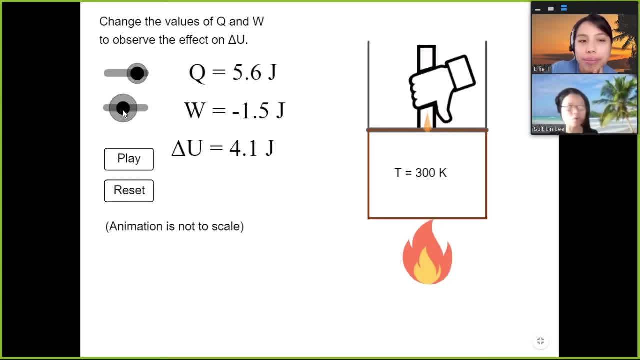 We add heat and then we also compress. Oh, we can pull up, Go all the way. I think we go positive first now, Okay, okay, okay. So we add heat and we also compress. So you see, wow, 5 plus 2.4 can increase internal energy. 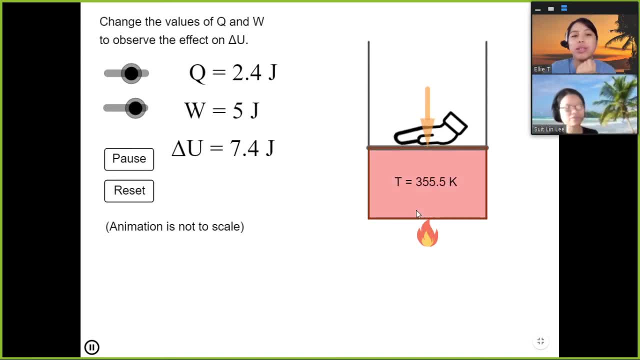 So you see, lor, you play, So you're adding heat, but you're also compressing, so the temperature will increase. Because the temperature is increasing, your internal energy is increasing. Yeah, so you can see from the number and the distance What if we go on the negative scale. 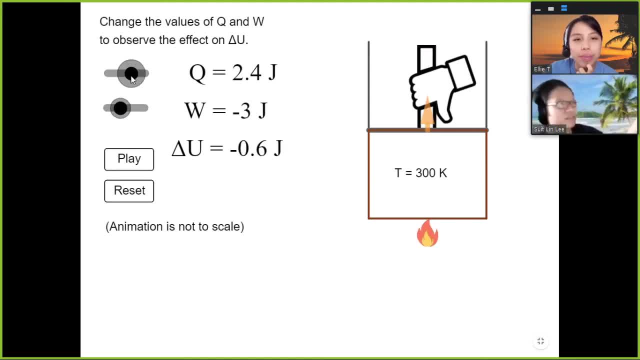 So we pull la, Make the gas bigger, Okay. so let's say we put Q at zero, Hmm, Okay. Wow means can have negative value. one, ah, internal energy. You see, the delta. The delta is for change guys. 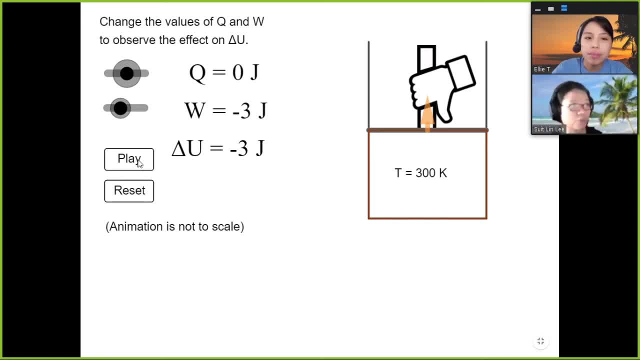 So when the delta is negative, it means that the internal energy decreases, Which makes sense because you expect the particle to slow down So you can see the temperature decreased to 277.5.. Then you can also do one where you remove. Yeah. 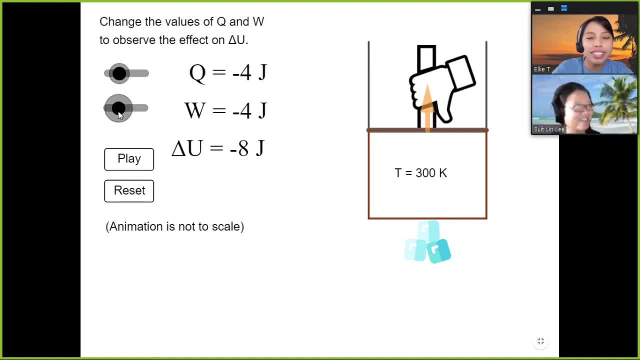 I guess they put ice cube to show that you remove heat But also you expand. you force the gas to expand, You do work, done Yeah, By gas. So the temperature will drop very fast, Because now I need to throw out heat to the environment. 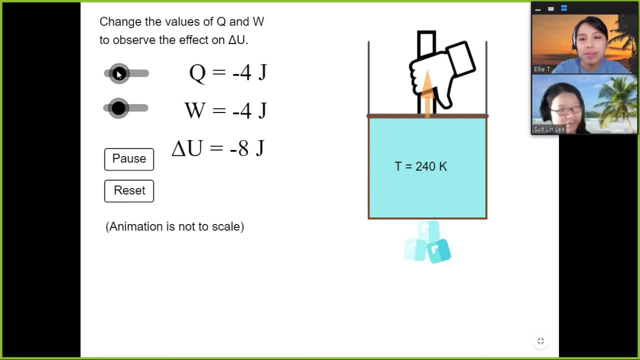 I also need to expand. This is called very tired, So the temperature decrease. I need to do many things Okay. So of course the sign convention here is important. It really depends on. So Q is positive When you add heat. 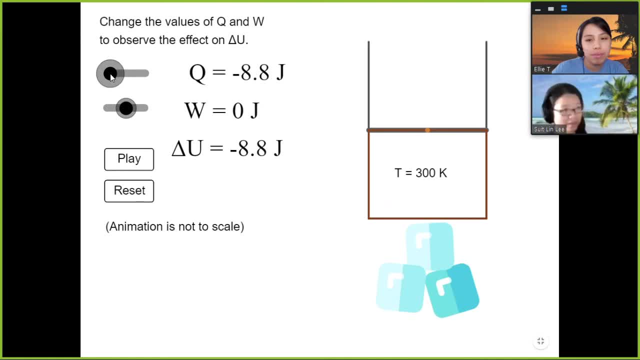 Q is negative When you remove heat, In this case represented by the ice cubes, Alright. W is positive if the piston expands, So if we play Sorry. W is positive if the piston compresses, You press down, You do work. 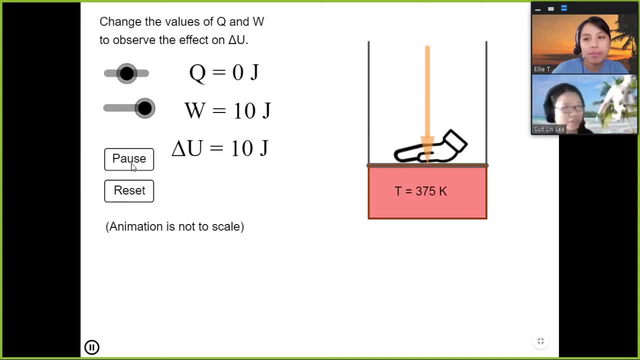 Yes, You play this, You will see. Oh, it is being pressed down. So W is positive when it is being pressed down And then W is negative When it is being pulled up. Okay, Good to know the sign convention. 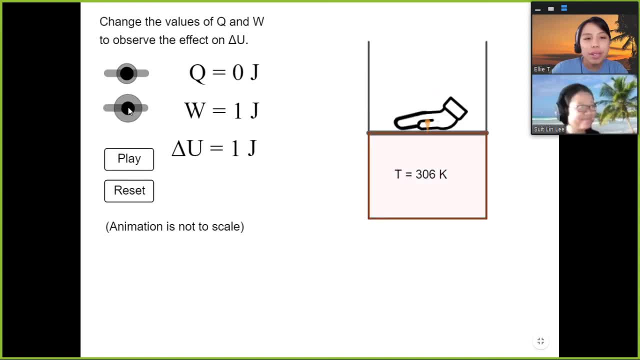 What about the delta U? Hmm, Delta U looks like when positive, you increase the delta U. Hmm, So delta U is positive. Negative means you decrease the delta U. Yes, So the tell to know whether delta U is positive or negative. 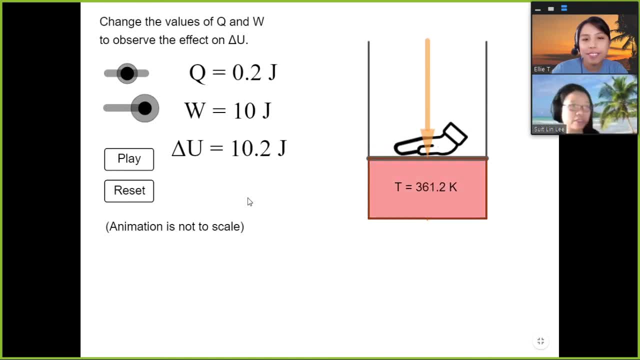 The clue that you can get from a question or a scenario is the temperature. When the delta U is positive, You see, it is higher 361.2 compared to 300.. And if delta U is negative, It is lower 241 compared to 300.. 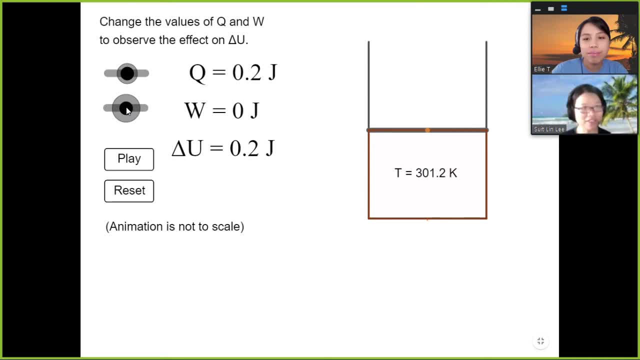 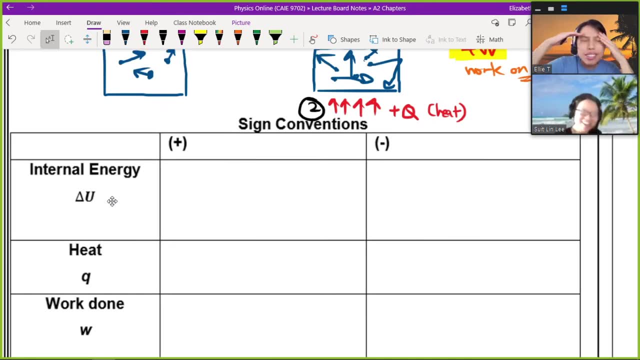 So we will summarize all of this in a table now. So let's go and look at that table. This one will save your life during exams. No lah, It will help you group the info in your head. Otherwise you will be like how positive, negative. 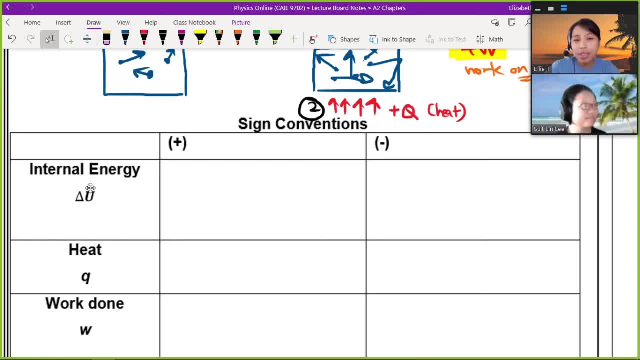 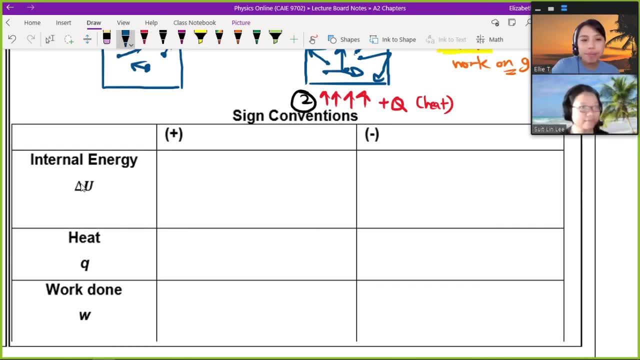 Miss how I confusion. So make sure you write this down somewhere in your notes, in handout or otherwise. Okay, So Miss. what is the sign convention we observed just now? The internal energy increases If delta U increases If delta U is positive. 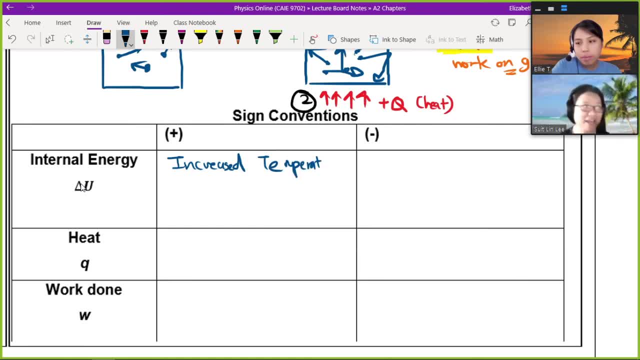 And the physical or the macroscopic tell is that the temperature increases. So increased temperature leads to increased internal energy, Because you know internal energy is 3 over 2 NKT. So increased internal energy and your delta U is positive. Okay, So the converse will happen. 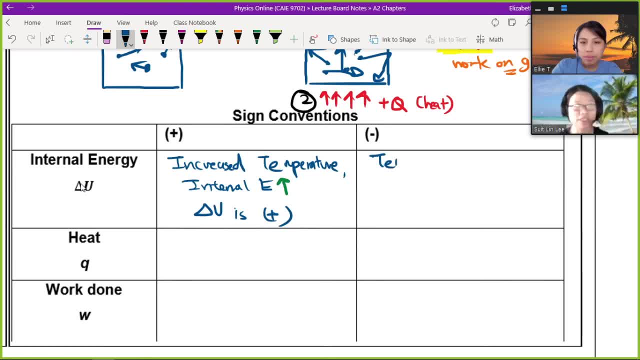 When you talk about the negative sign, We decrease the temperature. So temperature increase or decrease does not really depend on whether heat is added or not. So this is the part that sometimes confuses people, Because we are so used to thinking that if the temperature increased, then heat add. 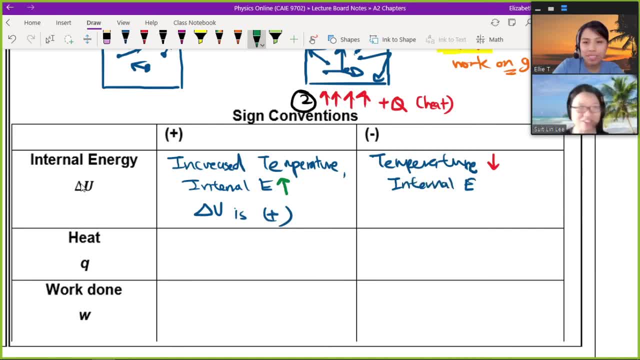 Temperature decrease, then heat remove. I don't know. I just want me to see the volume got changed or not and how the volume change. So it depends, Okay. So in this case, the only thing that you can say when the temperature changes is the internal energy. 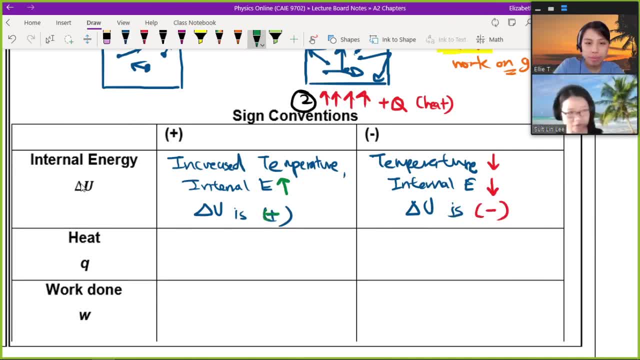 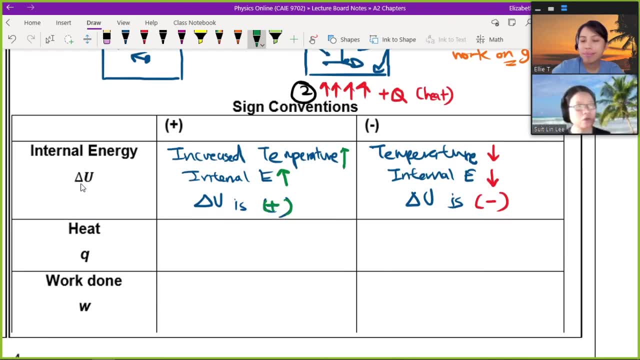 Temperature: increase internal energy. increase positive delta U. Temperature: decrease internal energy, decrease negative delta U. Heat is very straightforward: You add heat to the system. Heat added, Then plus Q, Q positive, Q positive, You add heat. 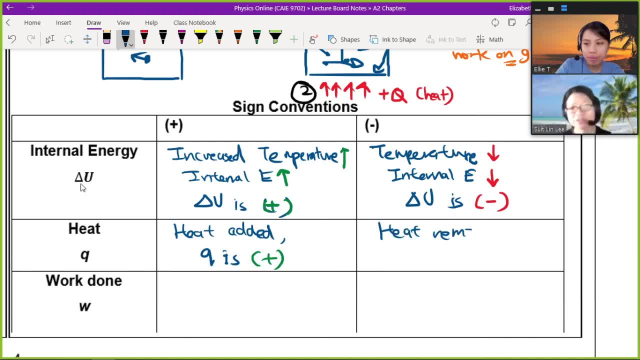 Q: positive: You remove heat. Negative: Please don't write put ice cube. If I see put ice cube in your answer I will laugh. It will be very entertaining and I just give zero. Put ice cube. Say heat is removed. 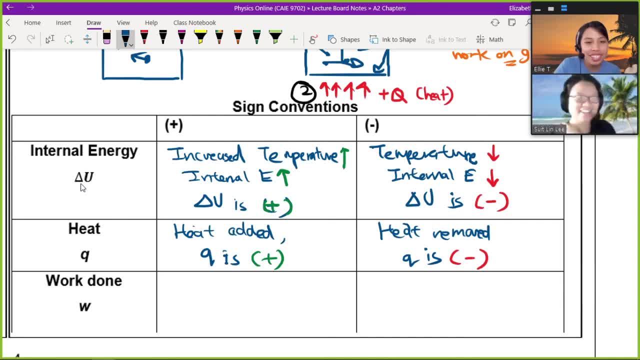 The ice cube is just a simulation for you to see. I guess if you wrap, you, tap out the whole thing in ice, you can remove heat If the temperature is different. But please just say heat removed. Okay, Here is the part that can be a bit of a jump. 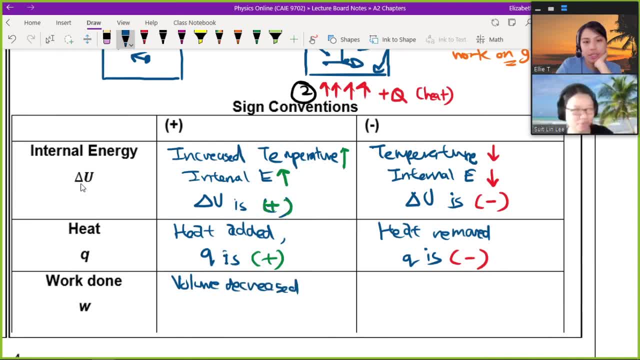 Because this one all increase. You can brain, But work done In order to increase the kinetic energy is volume decrease. Why like that? Because CIE chose this equation. So this is the same connection. Okay, So gas is being compressed. 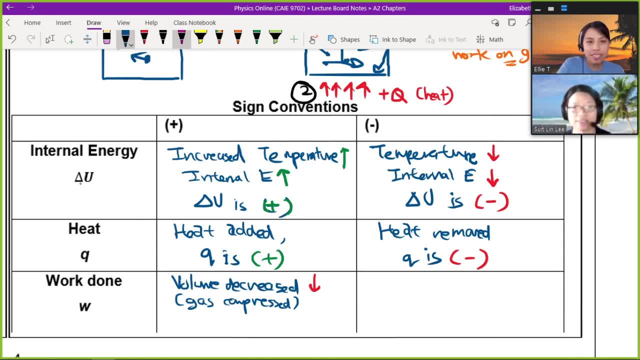 This is work done on the gas, Work done on gas. So it becomes smaller. So you work on the gas And the gas receive your energy with thanks And its internal energy will increase. That's why delta U is Q plus W. 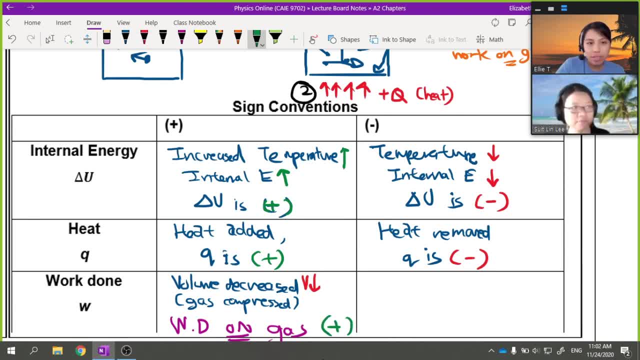 For the positive portion, Then for the negative portion. The negative portion- your volume will increase The work done one. you have to pay a little bit more attention now, Because the sign is kind of reversed in some of your brains. So when volume is increased, it's work done by the gas. 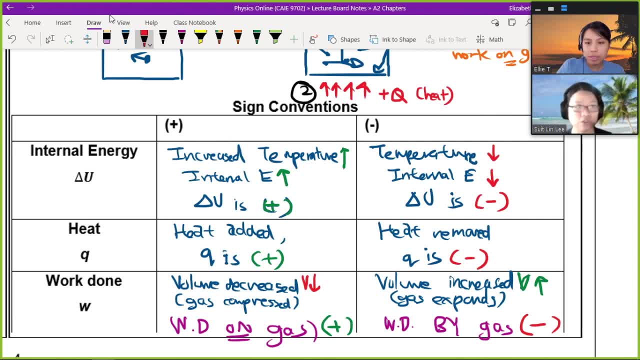 So when the gas do work, it will lose its internal energy. You do work, then your internal energy decrease more. So next time when people ask you: how are you? My internal energy is very low. I do too much assignment Microsoft Teams every day.